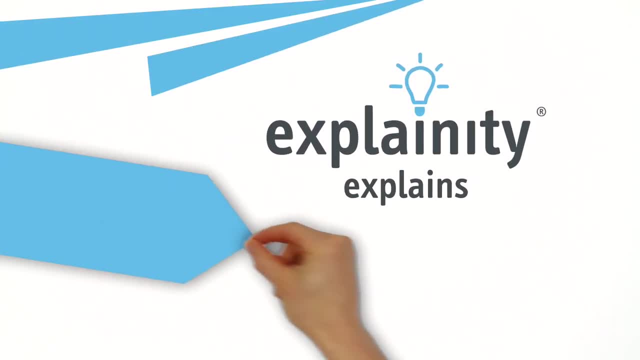 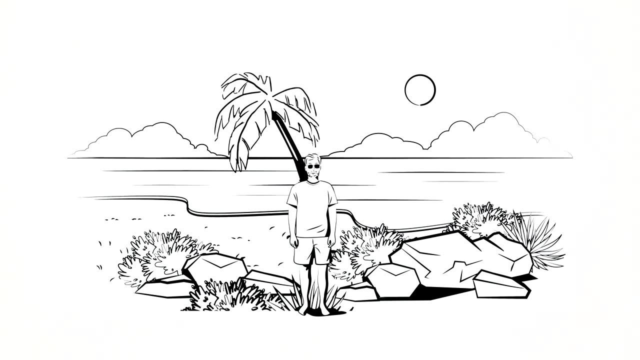 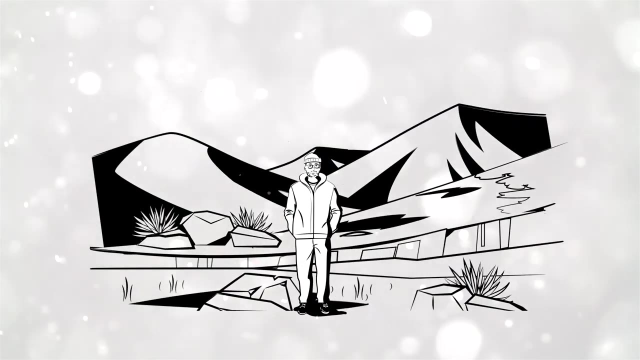 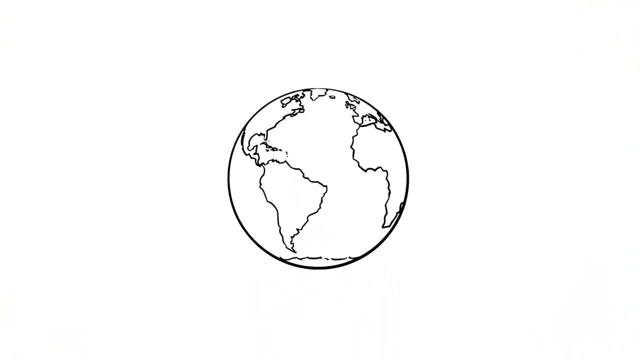 Heat around the equator, hot summers in the Mediterranean, spring, summer, fall and winter in New York, snowstorms in Greenland and icy temperatures at the South Pole. The global climate can be divided into multiple zones. Here a range of factors come into play. 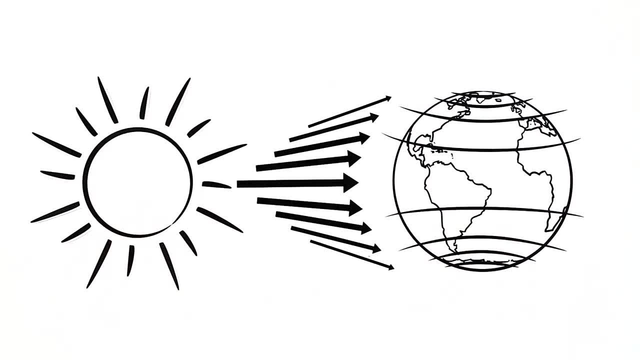 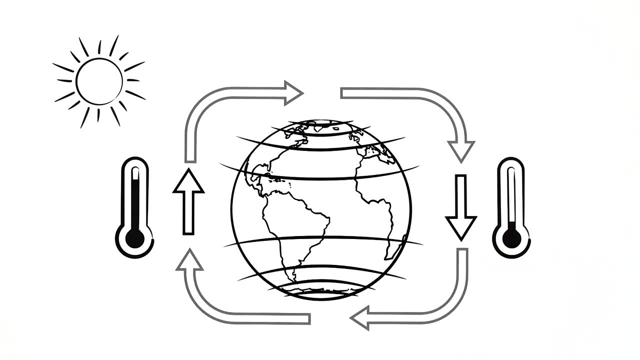 Among the most important is the sun. Depending on the position of the earth relative to the sun, it heats the land and water more in some places and less in others. In this process, warm air rises while cold air sinks. This results in wind, water vapor and rain clouds. 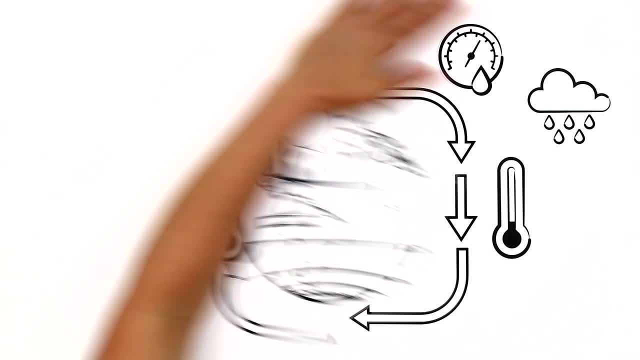 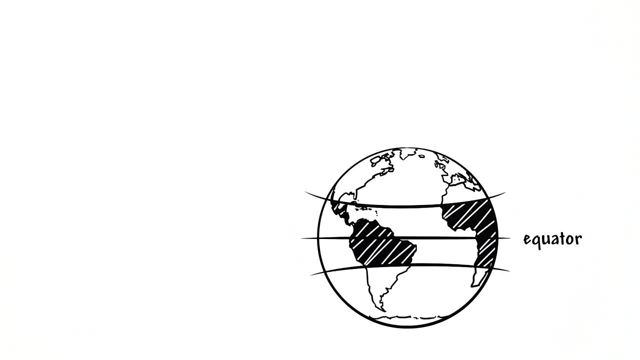 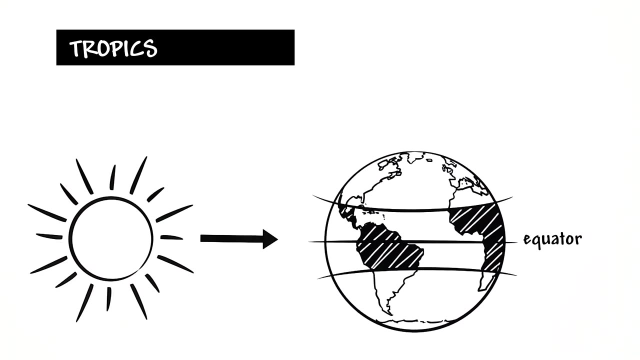 All this contributes to climate distribution. There is a line around the Sun in the center of our globe called the equator. The regions surrounding this line are the tropics, Since the sun's rays hit the earth here almost straight on, all year round. 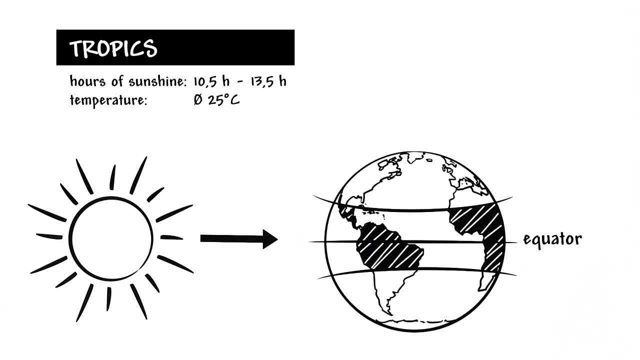 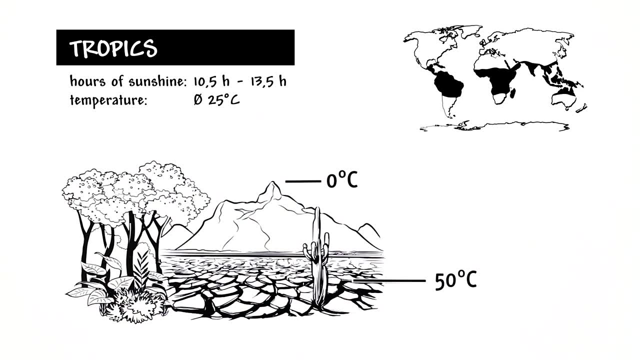 days are basically the same length and also just as warm, whatever the season. Depending on the altitude. temperatures range between 50 and 0 degrees Celsius. The tropics are home to rainforests with lots of precipitation, where plants grow in abundance. 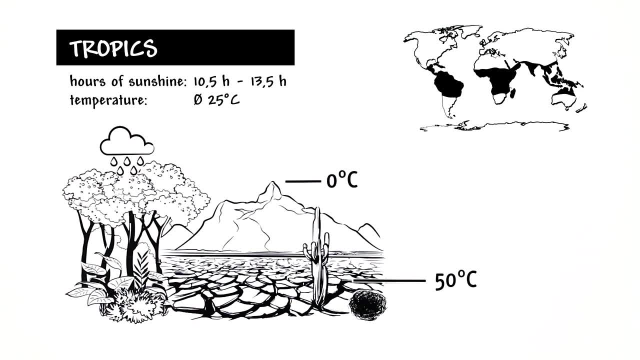 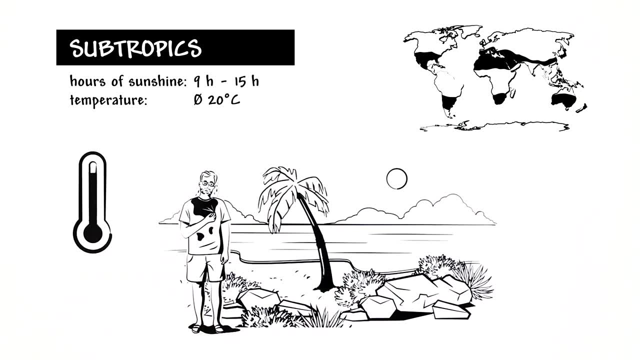 as well as extremely dry regions such as the savannas in Africa. Adjacent to the tropics are the subtropics. The summers are very hot, but the average temperature of the coldest month remains below 20 degrees Celsius. The subtropics include a number of deserts. 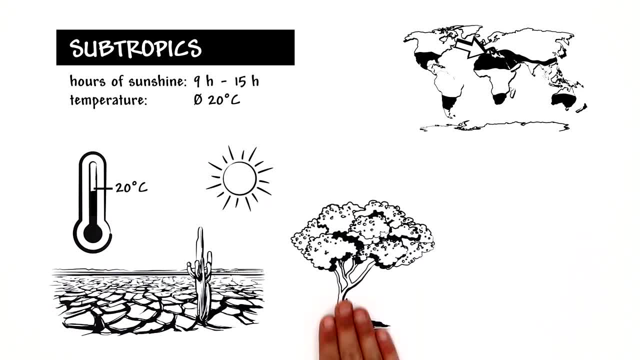 as well as the Mediterranean region. Here the summer months are relatively dry, While in winter plenty of rain makes the landscapes flourish. And then there are also regions where every month brings scattered showers. Different plants flourish here at different times of the year. 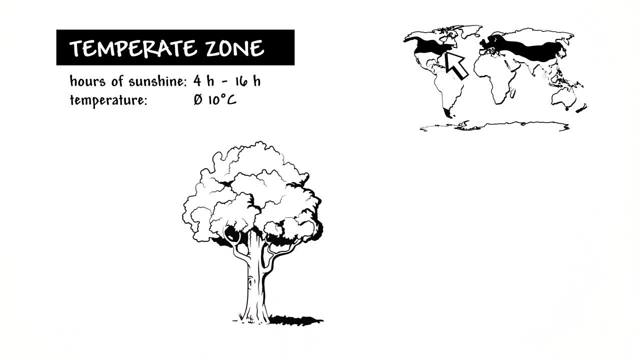 The temperate zone, which includes New York, is defined by the familiar seasons. Winters can be icy, cold, with a maximum of four daylight hours in some areas. On the other hand, summers are pleasantly warm, with up to 16 hours of sunshine.